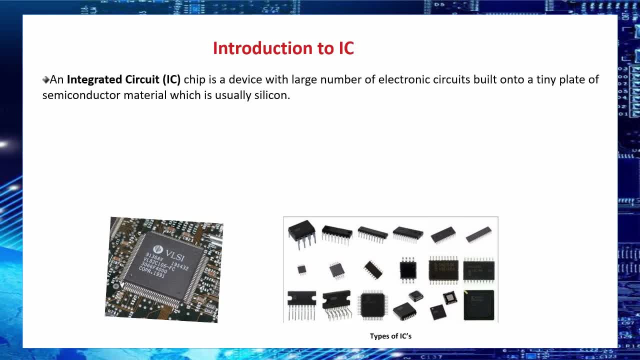 components built onto a tiny plate of semiconductor material, which is usually silicon. So, based on the number of components per chip and its complexity, IC generations emerged from small scale integration, medium scale integration, large scale integration to very large scale integration. So a VLSI IC is where millions of electronic components like 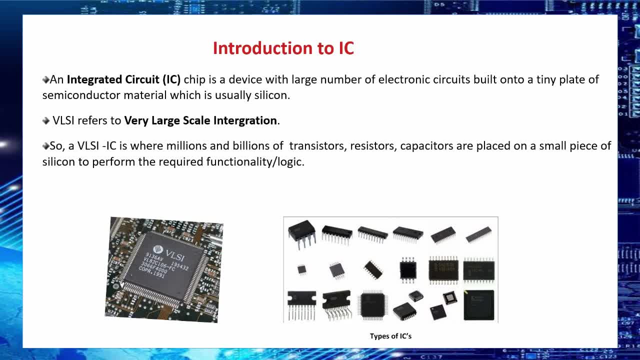 transistors, resistors, capacitors, are placed on a small piece of silicon to perform the required functionality or logic. Many applications include the microprocessors in PC, laptops, mobile phones, chips in the graphic cards, digital cameras, automatic cards, etc. 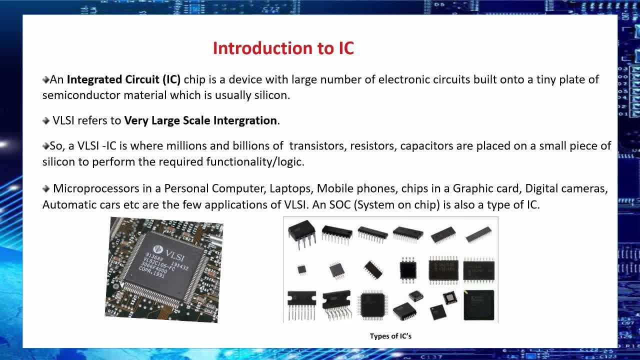 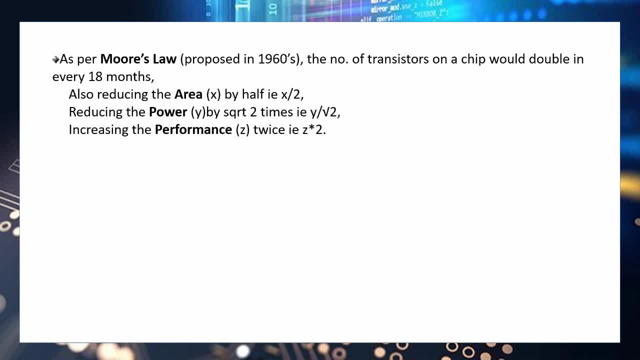 An SOC is also a type of IC. As per Moore's law, the number of transistors on a chip would double for every 18 months, also reducing the area by half, reducing the power by square root 2 times and increasing the performance by 2 times. 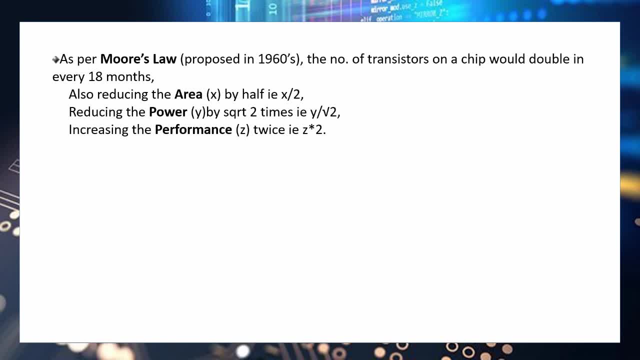 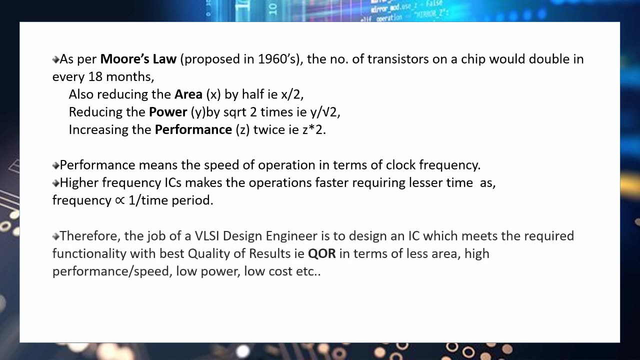 Performance means the speed of operation in terms of clock frequency. Higher frequency ICs makes the operations faster, requiring lesser time, as frequency is inversely proportional to the time period. Therefore, the job of a VLSI design engineer is to design an IC which meets the required 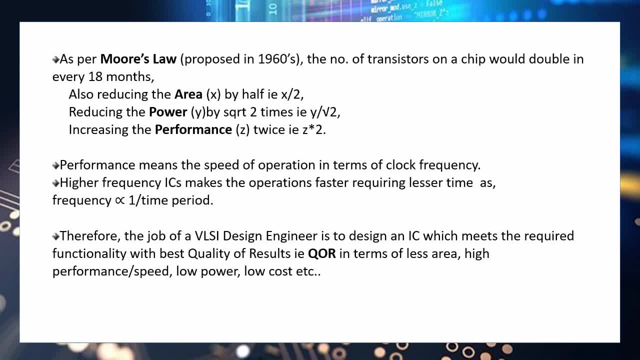 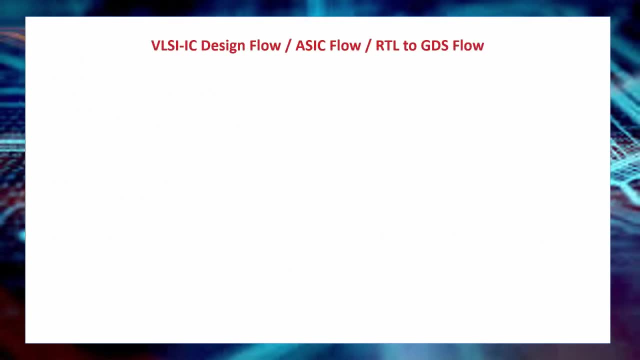 functionality with best and optimized quality of results in terms of less area, low power, low cost, high performance. Now let's see the overview of the flow involved in a digital VLSI IC design or ASIC design. ASIC in the sense Application, Specific IC. 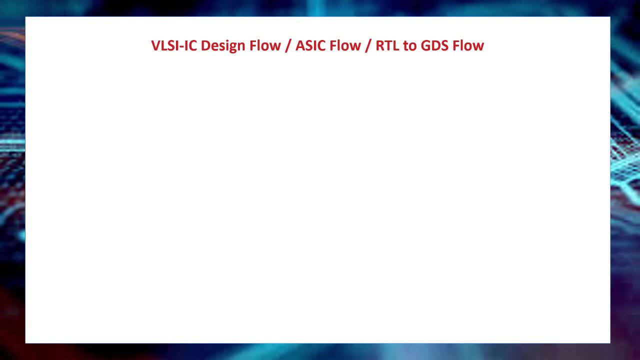 Like IC design for a laptop is one application and IC design for a mobile phone is another, The chip designed for a particular application is ASIC. Now the design flow starts with a given set off, As per the given specifications or requirements or the features that our chip must possess. 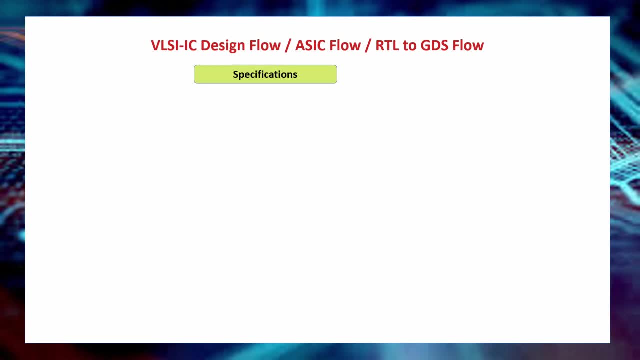 ie in terms of functionality, means what logic or function it must perform, how much area it must consume, with what clock frequency it must operate, what must be the area of the chip, etc. As per the given specifications from the customer, the top level engineer designs the architecture. 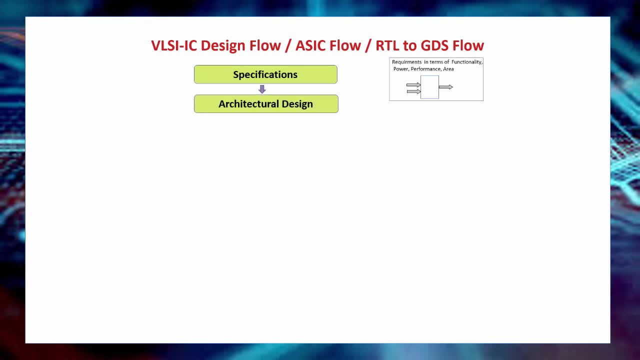 of the chip in the form of block diagram, ie what must be the different blocks that are in the chip and where the design must contain, etc. and its interconnections. The cost of the chip is also estimated at this stage and if everything is fine, then 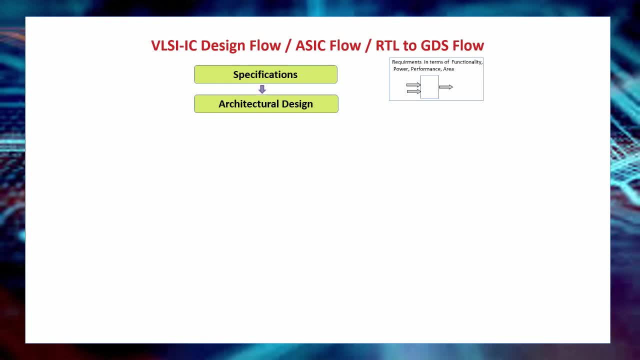 it is proceeded to the RTL design. As the ASIC designs are very complex, EDA tools are used to proceed Now, from the block diagram or the architecture, the RTL engineer derives heavier or function of the design in an algorithmic manner. Yes, we will discuss that in a minute. 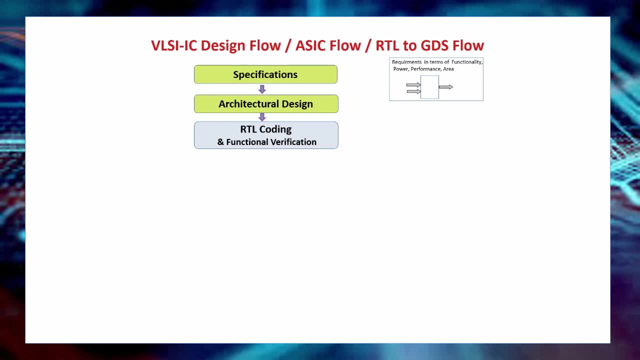 an RTL code using hardware description language which may be Verilog or VHDL, so that the code- RTL code- is understood by the tool. RTL is the register transfer level, which includes interconnections of the combinational elements, like logic gates, and the sequential elements, like registers, as per the functionality. Xilinx tools are commonly used for the RTL. 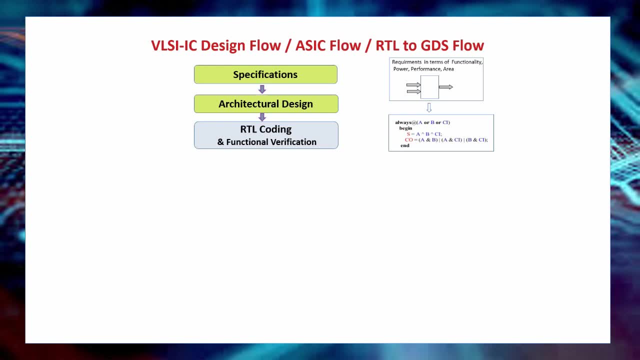 coding. it is coded using Verilog behavioral model. anyone who has the knowledge about Verilog coding can understand what is behavioral data flow and structural model in the Verilog behavioral model represents the algorithmic way of representing the behavior of the design. it also uses some mathematical or arithmetic expressions. now next step is the functional verification that. 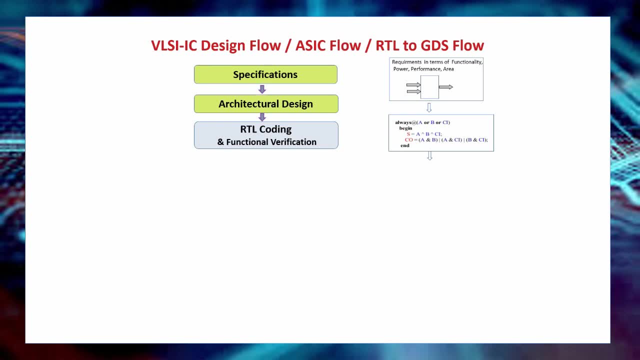 is to verify the code: Verify and cross check the RTL code whether it satisfies the functionality and the given specifications. if there are any errors, the code is modified and iterations are made until the specifications are satisfied. the next step is logic synthesis. in this stage, the tool converts the RTL behavioral model code into the structural Verilog code, which is: 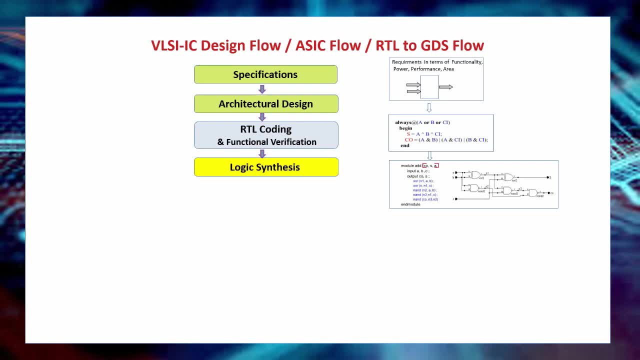 a gate level netlist. The tool used for logic synthesis is design compiler from synopsis or genus, from cadence. mostly inputs required for the logic synthesis are RTL code, library files and SDC constraints file. the logic synthesis happens in three stages: translate, mapping and optimize translate. 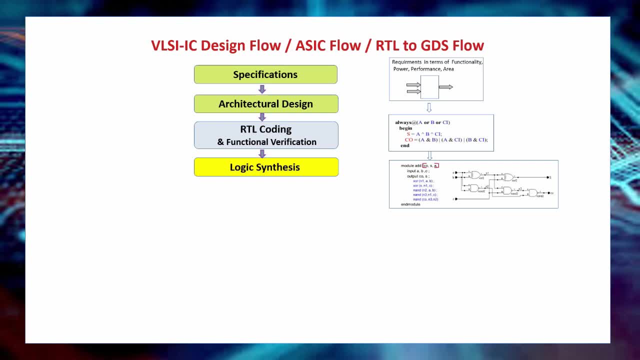 means the tool converts the high level RTL circuit into its corresponding logic gates. For example, like the full adder at higher level circuit representation is implemented at lower level of representation in the boolean logic using simply the logic gates. The functionality remains the same, however. 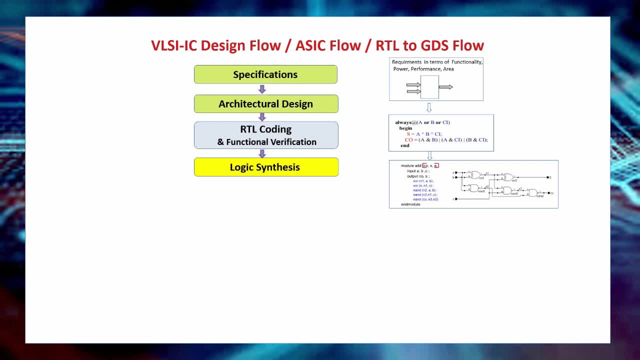 Next is technology mapping. here the tool maps the logic gates with the required technology that we are designing in, that is, in where, whether in 28 nanometer or 14 nanometer or 17 nanometer, etc. The next, the next, is to optimize. the tool does optimization in terms of power area, timing. 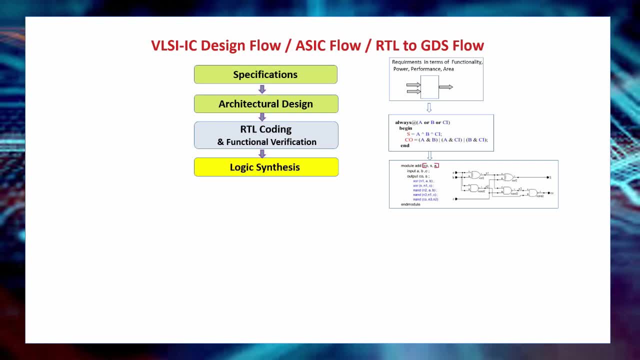 and that is to get the best QOR. Then design for test, that is, DFT insertion, is also done at this stage by the DFT team. Now the gate level simulation, that is, logic verification and testing, is done. We check whether it performs the required logic and iterations are made until there. 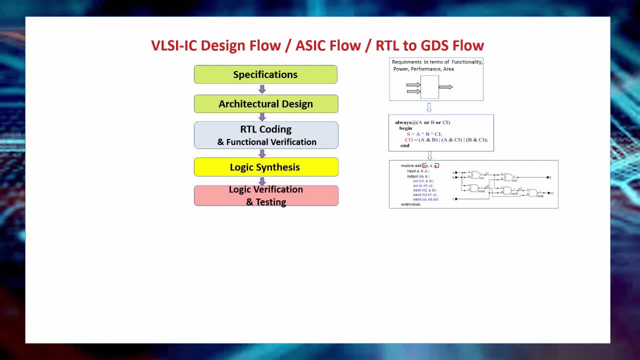 are no errors. The output of logic synthesis are gate level netlist and SDC constraints file which are given as input to the physical design. The tool used for the physical design are mostly ICC2 by synopsis, or Innovers by cadence. So that's it. 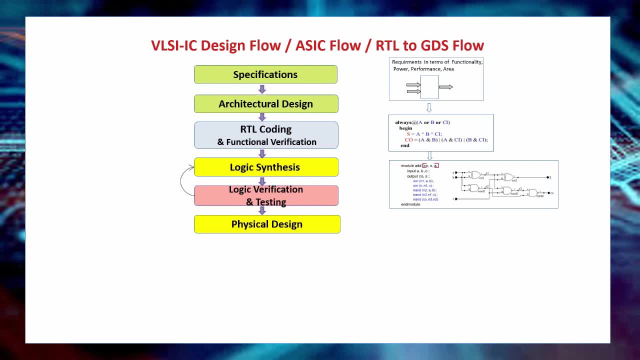 In physical design or PNR. the gate level netlist is converted to the GDS format. GDS is graphical database stream. It is nothing but a transistor level layout format that is the physical representation of our design, which can be manufacturable. The various steps involved in PDR design import, where all the inputs are read by the tool. 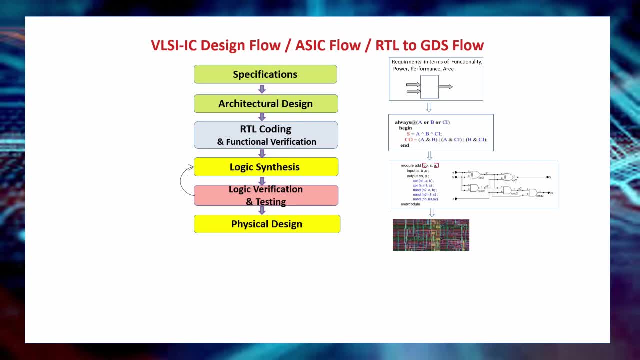 floor planning, power plan, placement, CTS and routing, with optimizations in each stage. We will discuss in detail about each of these concepts in our next videos. Thus, in PD, gate level netlist will be finally converted to a GDS transistor level layout. 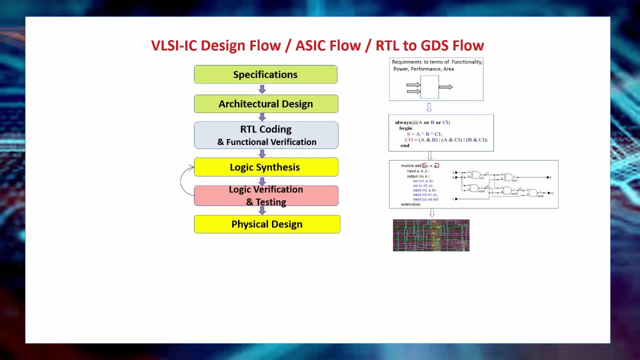 with best QOR, As we are familiar and have knowledge of implementing the logic gates like AND, OR etc. using the CMOS transistors, So the same concept follows here. Thus we can say: an IC consists of millions and billions of transistors, as the higher 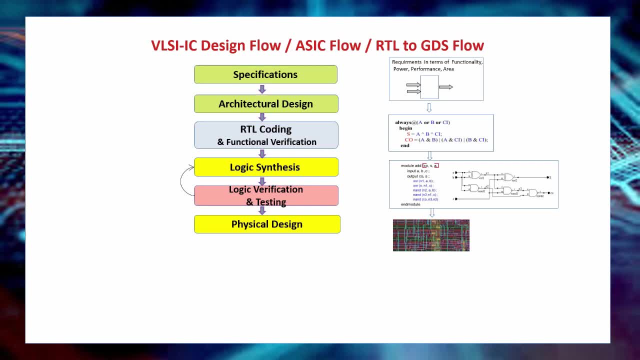 level circuits are converted and implemented using the CMOS transistors. Now the obtained GDS transistor level layout file is sent for verification and sign off. where different checks are performed, like design rule check, electrical rule check, LVS, timing analysis, Power analysis, 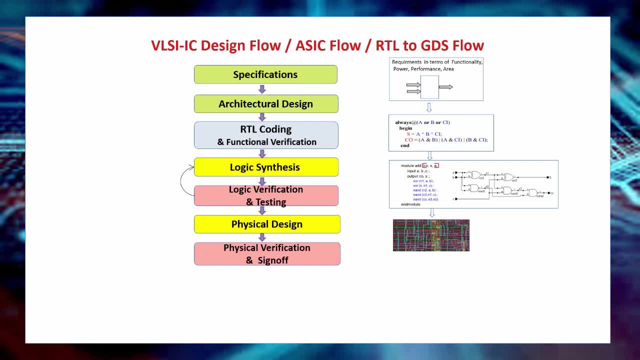 Cross stock analysis, etc. Then iterations and modifications are made until we meet the requirements. The GDS file after verification is sent to the foundry and this process is called tap out. In foundry the mask is generated for a design layout and chip is fabricated. 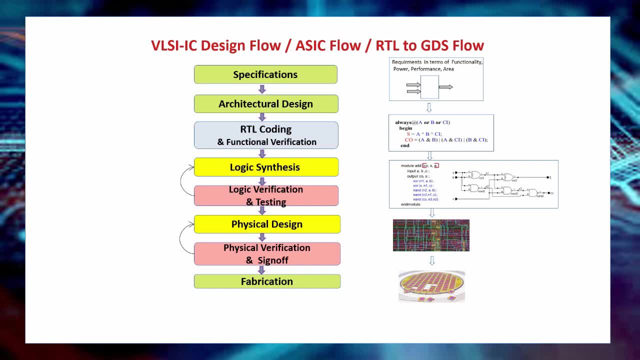 The fabricated chip is then packaged, THANK YOU, to protect from the external damage and again tested for any bugs before releasing into the market. After the final testing process, the bug free IC chip is released in the market. finally, This completes our IC design flow, or ASIC flow, and also called as RTL to GDS flow. 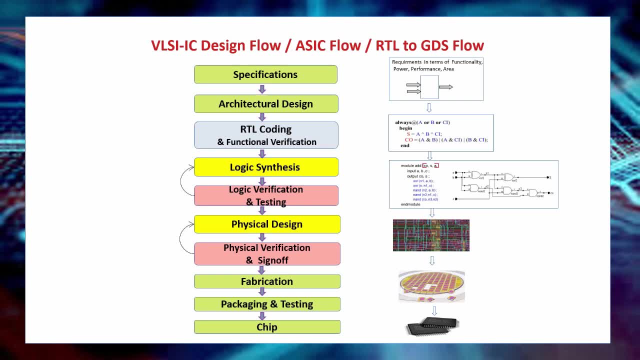 As we have seen, as the RTL code is converted to the GDS layout, which is physically manufacturable, The RTL design comes under the front end logic synthesis and physical design comes under the back end design. Thus we can say: VLSI IC design includes front end design and back end design. 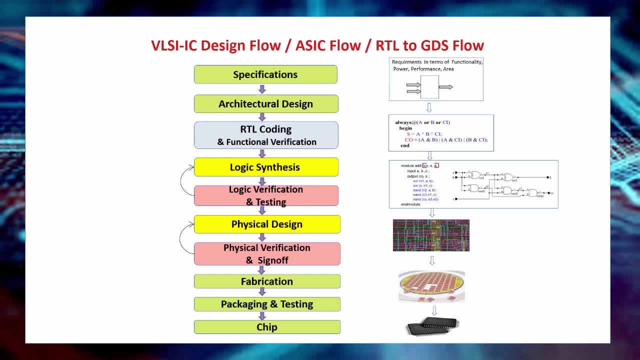 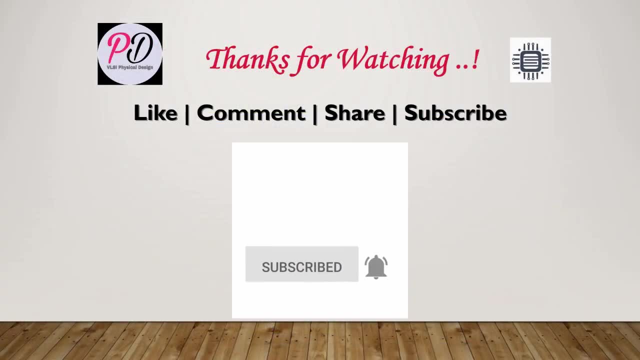 This is now all about the overview of ASIC design flow. For any doubts in this session, kindly comment in the comment section below. Thanks for watching.